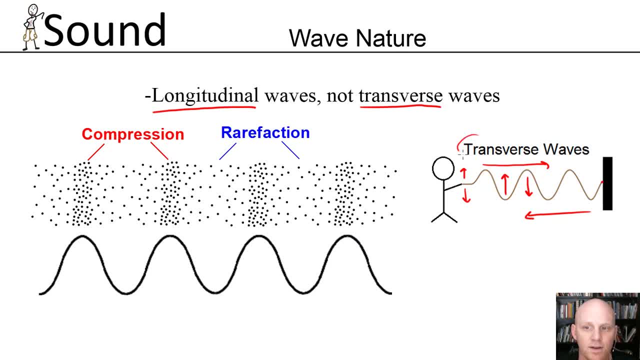 is perpendicular to the directions of propagation. that's what is meant by a transverse wave, And that is what a sound wave is not. A sound wave is a longitudinal wave, and in this case the direction of propagation and the displacement of the medium are in the same. 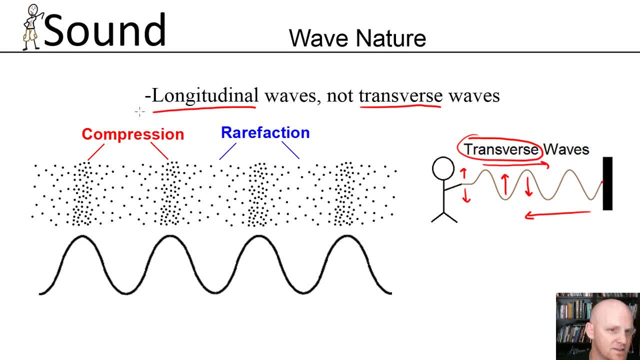 direction for a longitudinal wave, and that's what's happening here with sound. So let's start by taking a look at sound being propagated through a gas, in this case, like air. So first of all, sound does need a medium. You can't propagate sound in a vacuum And in this case I'm just going to have S here be my source. 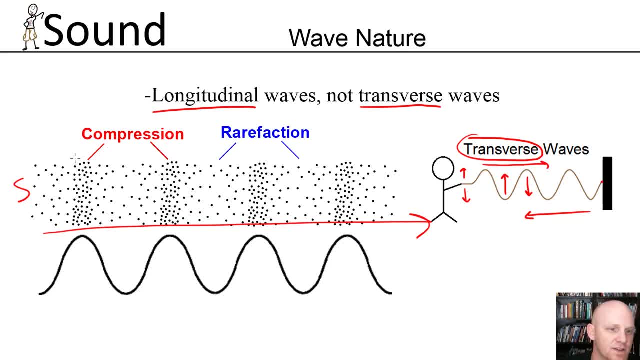 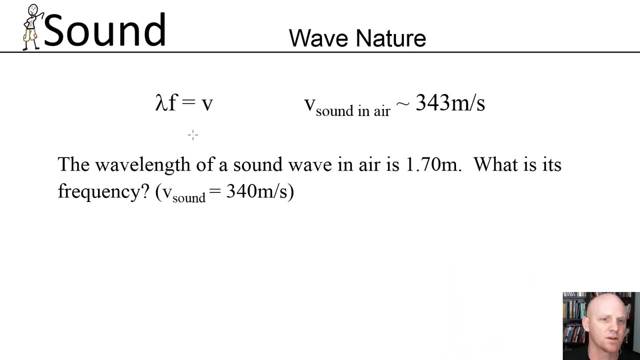 So sound, being composed of waves. we can look at these waves and they have a characteristic wavelength, represented by the symbol lambda here, as well as a frequency And, as is the case for any wave, the wavelength times. the frequency always equals the speed of the wave. 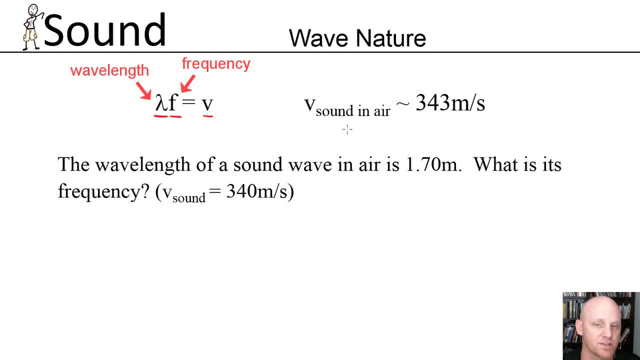 So in this case I've given you the kind of average velocity or the speed of sound in air. It's 343 meters per second. We'll find out in a little bit that it's actually temperature dependent, So this value is actually given at 20 degrees Celsius. 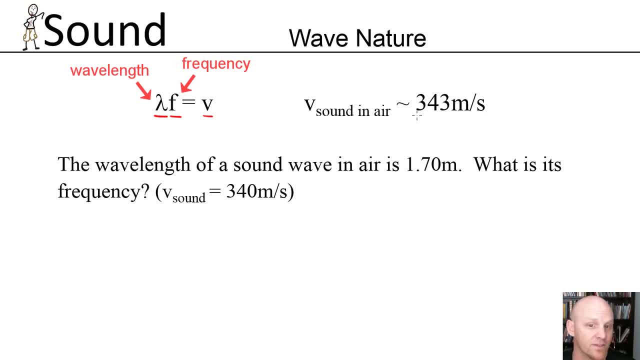 And a typical problem. they're going to have to tell you what the velocity of sound, even in air, is, because there's some variability there. So if we look here, there's three variables in this equation. Typically I've got to give you two and I can ask you to solve for the third. 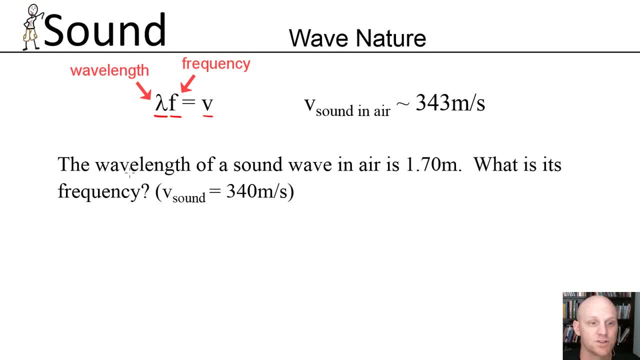 That's what this first question here down below is exactly doing. So here you're given the wavelength of 1.7 meters, You're given the speed of sound, at whatever temperature this is, So it's 340 meters per second. The question is: what is the frequency? 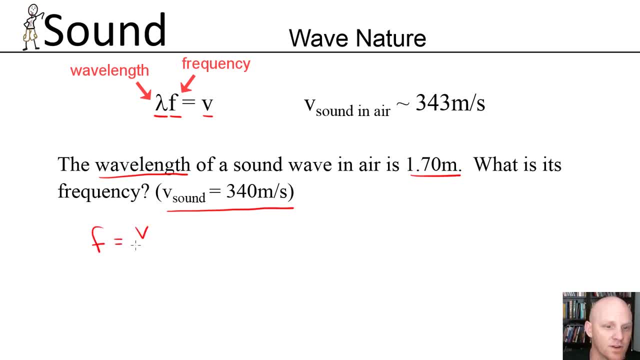 And so if we rearrange, we can see that the frequency is equal to the velocity of the wave over the wavelength, And so in this case that's going to be 340 meters per second over a wavelength of 1.7.. So, and if we do the math here, you can kind of see that 340 is the same as 3.4 times 10 to the second all over 1.7. 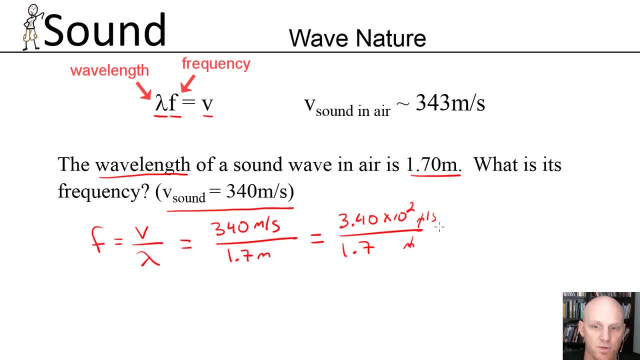 So notice the meters per second and the meters, the meters cancel, end up with 1 over seconds, which is the same thing as a hertz. So in this case, 3.4 over 1.7 is 2, and 2 times 10 to the 2 is the same thing as 200, and again 1 over seconds, or the same thing as hertz. 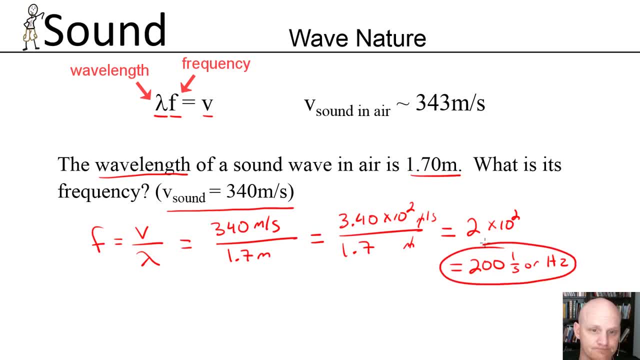 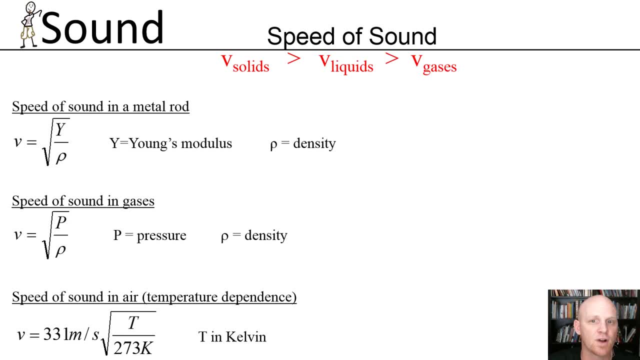 So there's your frequency: 200 hertz. So let's expound on our discussion of the speed of sound. The first thing I want to indicate is the difference between sound traveling in solids, liquids and gases. We find that in general, sound travels fastest in solids and then liquids, and then slowest in gases. 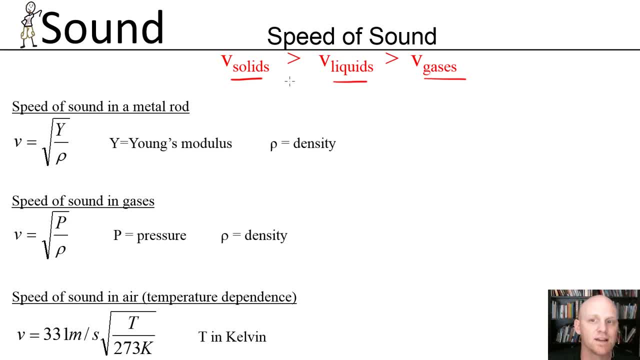 So you might know this from chemistry, but solids and liquids are much less compressible than gases And, as a result, sound propagates much more quickly through them. You may have noticed that sound travels much more quickly. It travels much more quickly underwater, so then it does above water. 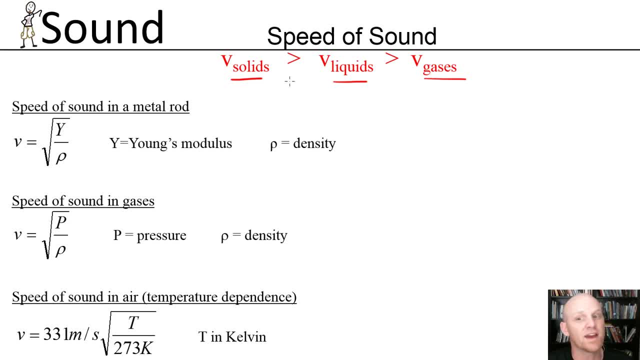 So when underwater, it's obviously traveling through the water, and above water it's traveling through the air, which is a gas. So a few relationships we want to specifically look at here is, first of all, the speed of sound in a metal rod. 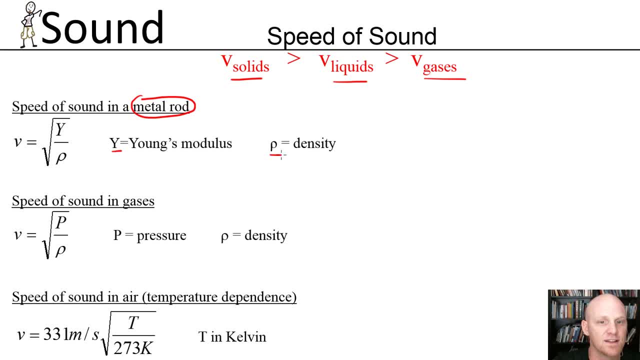 And it turns out it depends on two things. It depends on the Young's modulus as well as the density of that metal. So we see here that it is in some way directly related to the Young's modulus- Not directly proportional, but directly related. 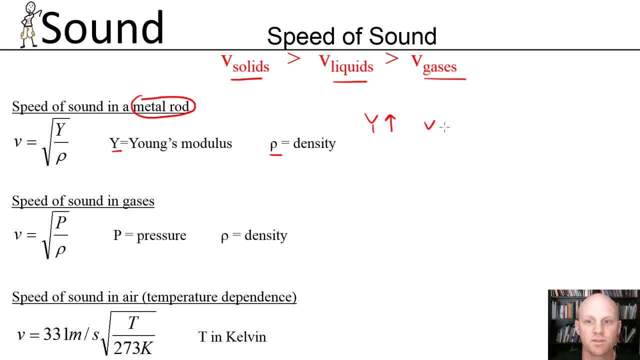 So as your Young's modulus increases, your speed of sound increases. It's also going to increase. But again, it's not directly proportional, just a direct relationship here. We see here that your speed of sound is actually proportional to not just your Young's modulus but the square root of your Young's modulus. 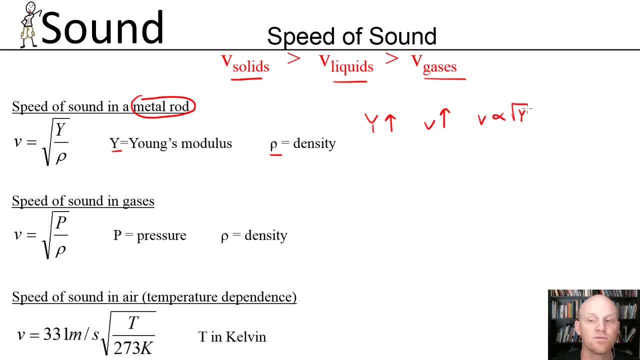 So therefore, to get a two-fold increase in the speed of sound, you'd actually need a four-fold greater Young's modulus from one metal to the second. We also see a relationship with density here. So in this case, density rho. as density increases, your speed of sound is actually going to decrease. 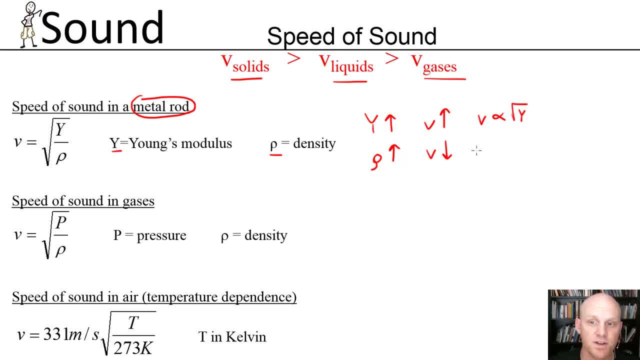 There's some sort of inversion, There's some sort of inverse relationship. They're not inversely proportional, but there is an inverse relationship. We see that your velocity of sound is proportional, not to one over your density, but to the square root of one over density. 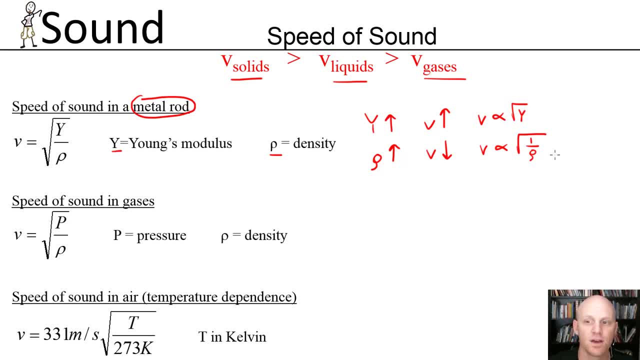 So here, if you wanted to get a higher speed of sound, you would actually have to have a smaller density, And in this case, to get a two-fold increase in the speed of sound, you would need a density that is four-fold smaller than your original metal here in this case, 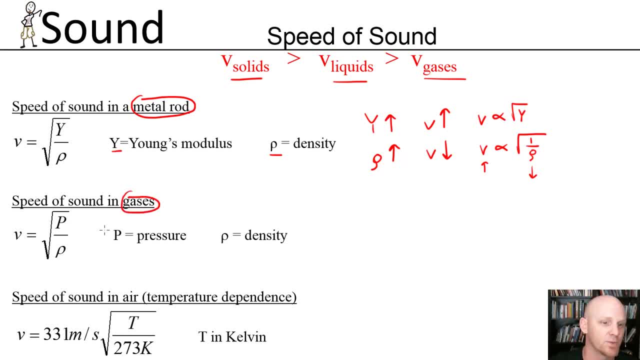 We can also take a look at the speed of sound, in this case The speed of sound in a gas. So there's a similar relationship Here. we find that the speed of sound in a gas depends on the pressure as well as the density of that gas. 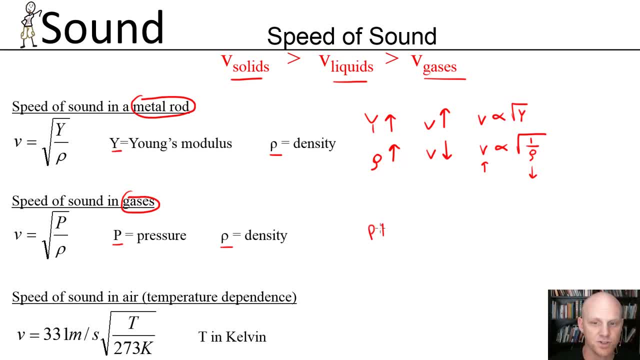 So when we see a direct relationship to the pressure, so again, as pressure goes up, your speed of sound goes up. But again it's not a directly proportional relationship, It's through the square root again. So velocity is actually proportional not to pressure itself but to the square root of pressure. 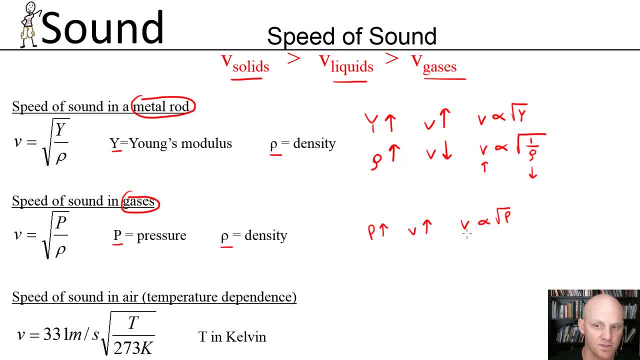 So again, a four-fold greater pressure only results in a two-fold increase in the speed of sound. We also see this inverse relationship again To the speed of sound. So as your density rho increases again, your speed of sound decreases. but it's not inversely proportional, just an inverse relationship. 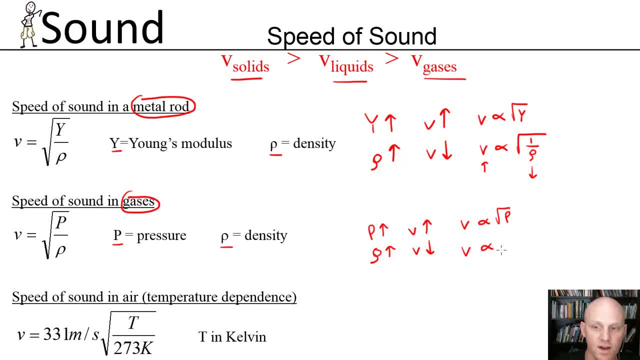 So again, velocity is proportional to not one over density, but the square root of one over density. So again, if you wanted a two-fold increase in your speed of sound, you would have to have a density of your new substance here, your new gas, that's four times smaller. 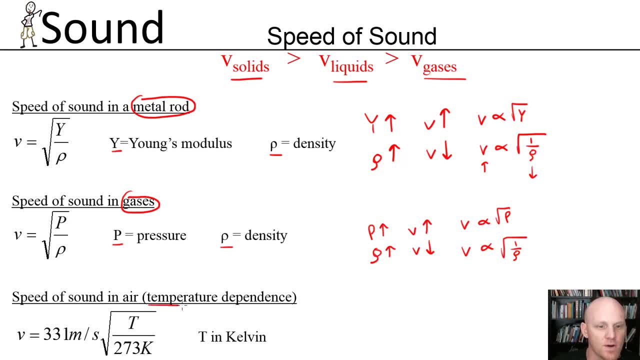 And finally, let's take a look at the speed of sound in air and take a look at how there's a temperature difference. So, and it follows this equation, this is the one I'm using, but you'll see in a couple different forms, some have a similar equation but where you plug in T in degrees Celsius, some use slightly different equations, but generally have some forms similar to this one right here. 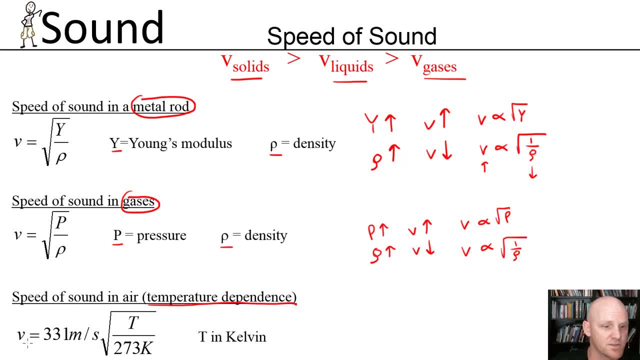 So if we look here as T goes up, we'll find that the speed of sound goes up, And if you plug in 293 here, you'll find out that your velocity of sound comes out to 343 meters per second, as we mentioned on an earlier slide. 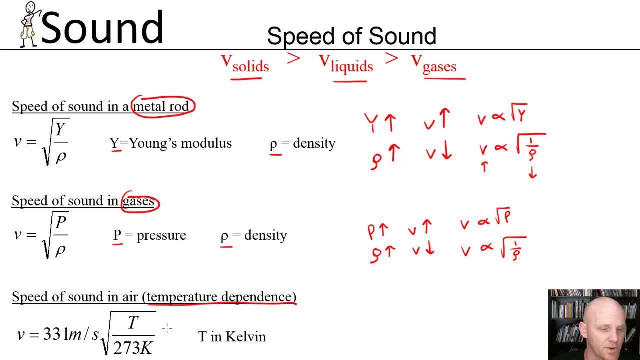 And basically it's just a plug-in function. Basically it's just a plug-and-chug way to figure out the speed of sound. but if you recall from your chemistry, knowledge with PV equals nRT, so that generally, as your temperature goes up, your gas expands. 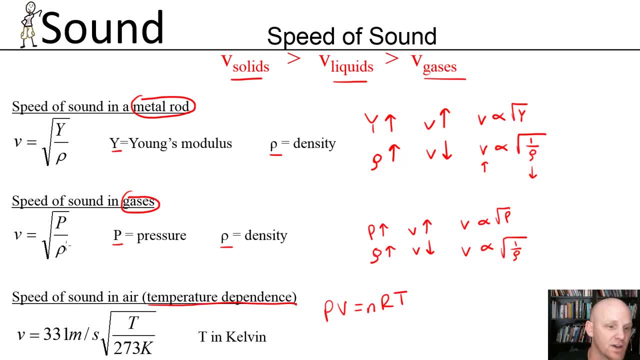 And as your gas expands, its density is going to become smaller. So, and if you get a smaller density, your speed of sound is going to go up, And so jives with what we learned in the last section here. so as temperature goes up, density goes down and your speed of sound also goes up as a result. 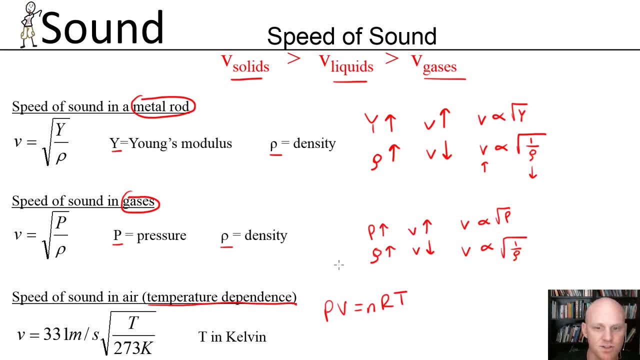 Now, with these three different forms, we're going to be able to figure out the speed of sound. Now, with these three dependencies, you may have some plug-in and chugging to do here, but you also need to understand these relationships as well.